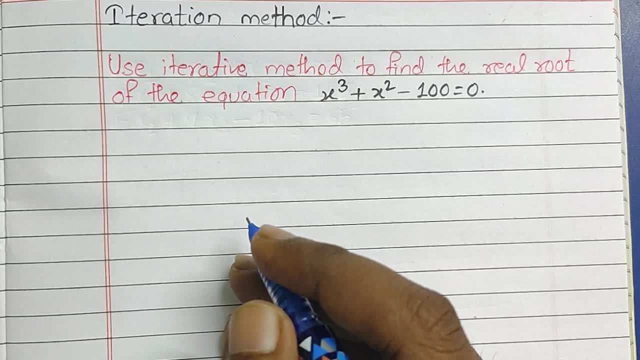 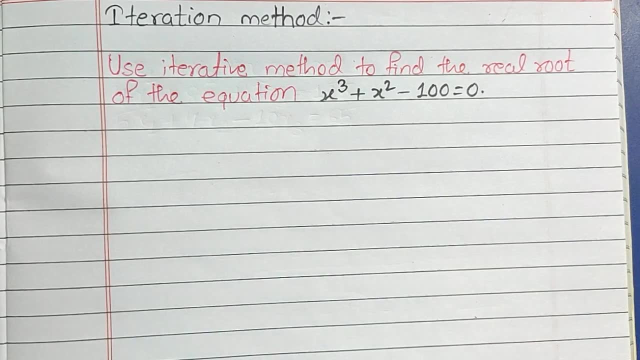 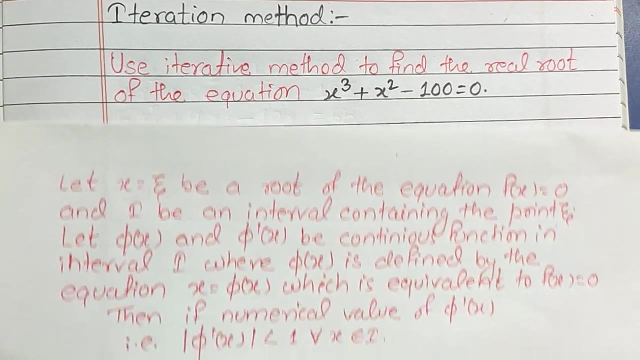 regular falsi method gives the approximate root, which is not exact, the real root. and without wasting time, let's begin the solution. and before beginning the video, I would like to give you the brief info introduction about the things which we are going to do in this video. first of all, as you can see, 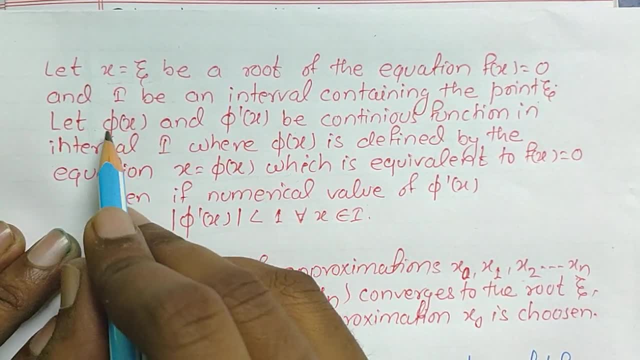 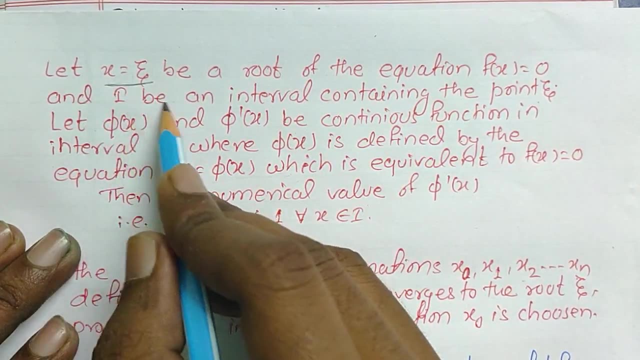 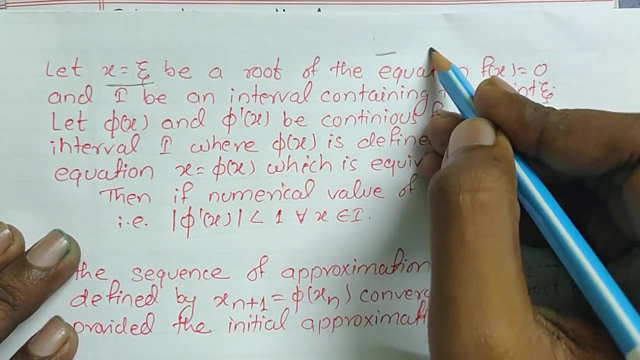 according to the concept of Newton-Raphson method. here it says that X is equal to Zeta is the root of the equation. FX is equal to 0 and I be the interval containing the point. Zeta means we we've here in this. while solving this numerical, we will find the integer like interval in which: 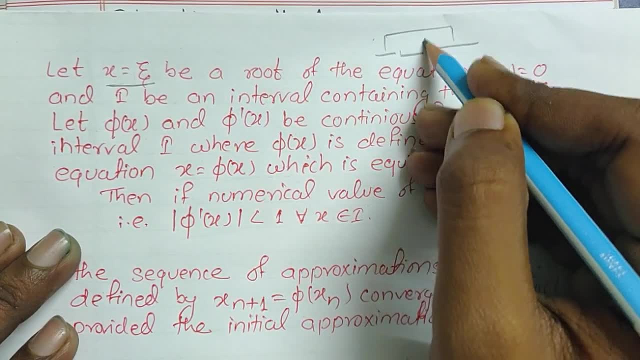 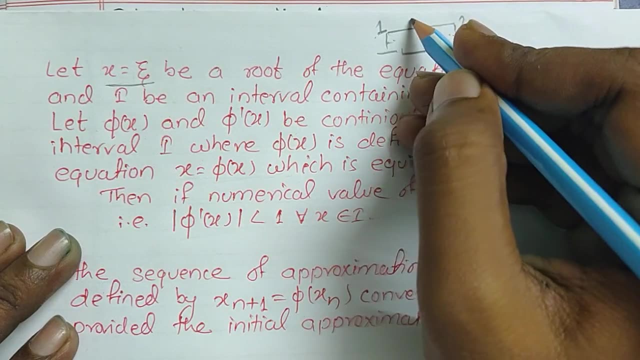 you and the our root or the panel of x will lie between that two animals suppose we have. we have find the root as 1 and 2, then our value, like 1.56 or something which will be the solution of x, will lie between these two. 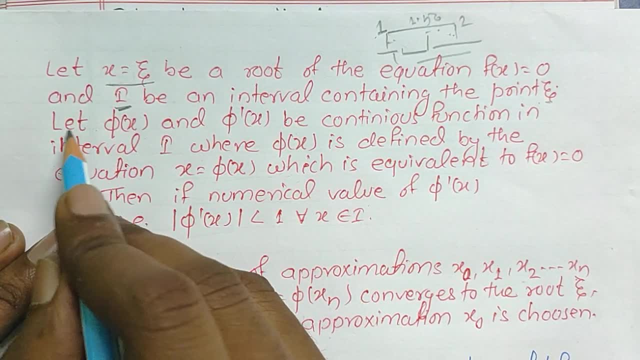 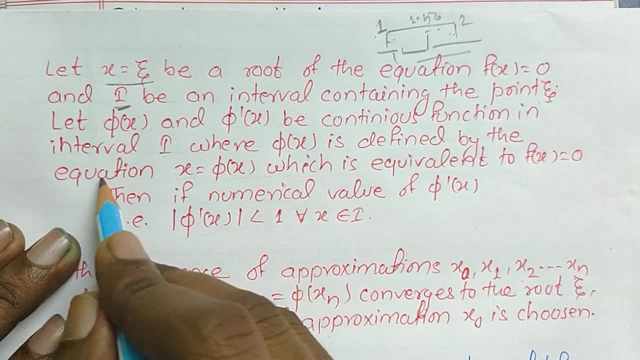 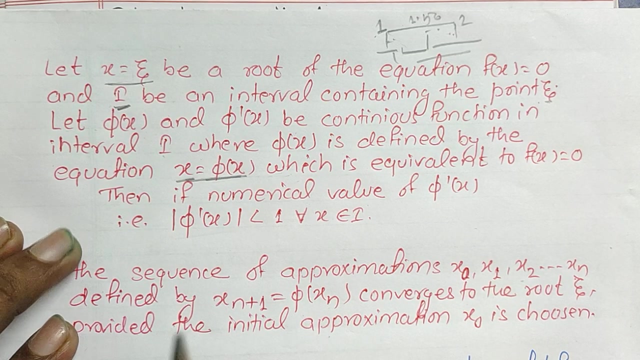 interval which is denoted by i, and for that let phi x and phi dash x be the continuous function in interval i, where phi x is defined by the equation x is equal to phi x. if any equation which which we are asked to find by solve, or solve by using the iteration method, we will write it in. 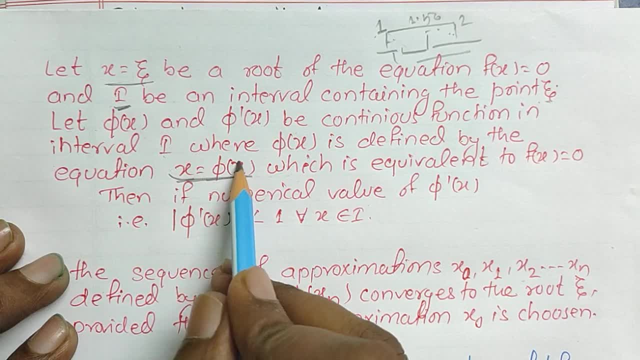 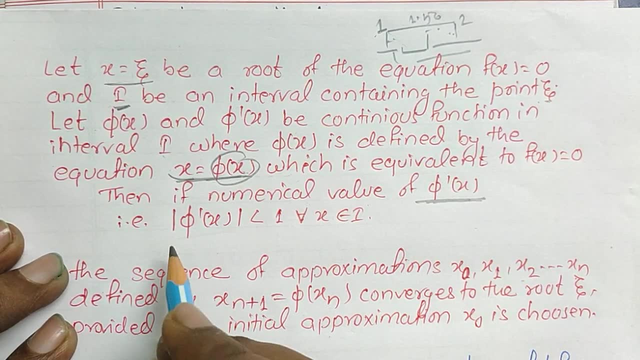 the form of x is equal to phi x, and then we will find the root of sorry derivative of phi x, which is denoted by phi dash x. and then the first condition for the application of the iteration method is that the modulus of phi dash x should be less than 1, and this theory will be more clear. 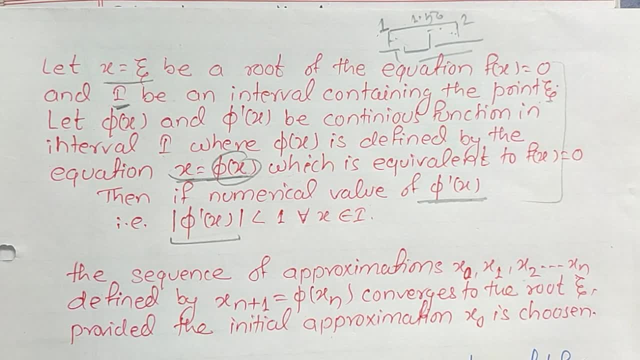 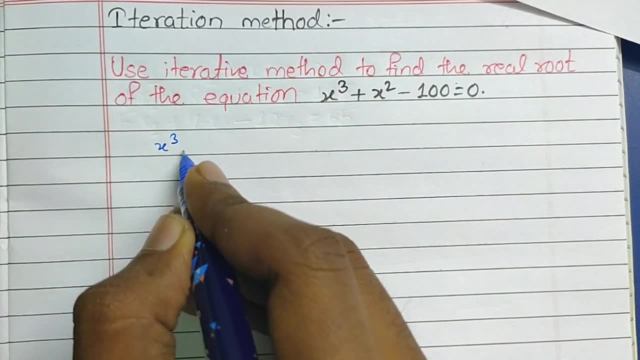 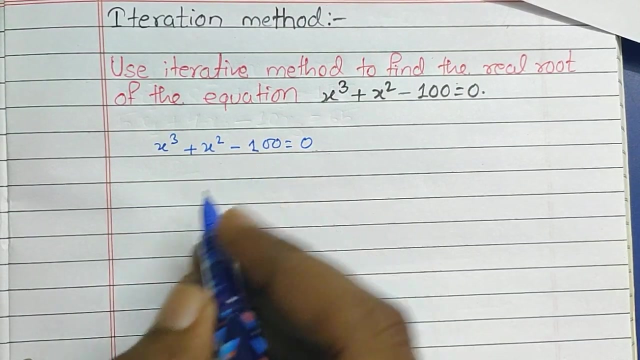 in this numerical. and so let's see how the numerical is solved. now, here you. we are, given the equation, which is x cube plus x square minus 100 is equal to 0. now, the very first step what we need to do is we have to write this equation in the form of x is equal to phi x, so 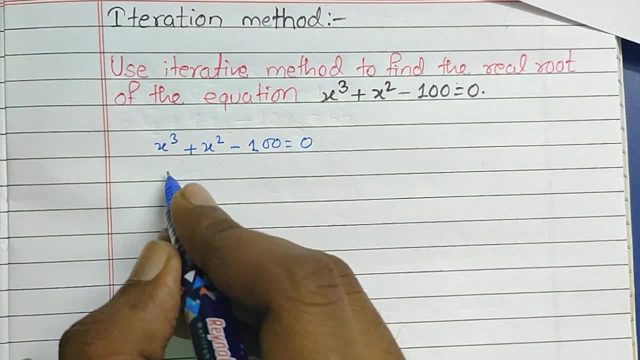 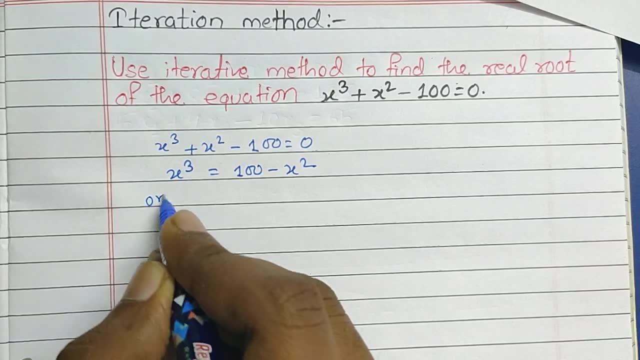 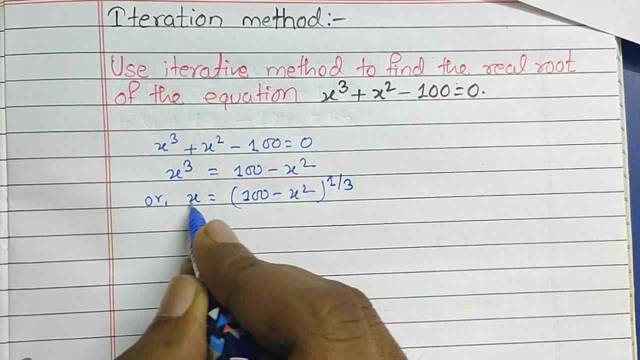 let's write it. then how we can write it, let's suppose. let us suppose this will be: x cube is equal to 100 minus x square. or x is equal to 100 minus x square to the power 1 by 3. now you can see that this is in the form of: x is equal to phi x. 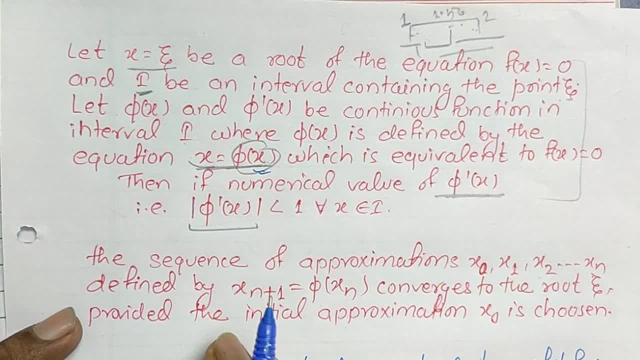 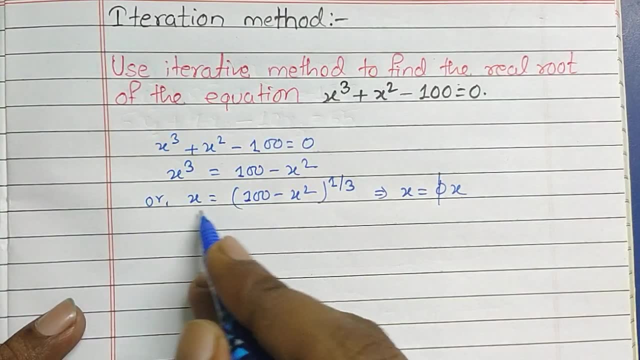 which the theory says means we have got this. now the second thing what we need to do is we have to find phi dash. x means derivative of derivative of this. derivative of phi x means we have to find its derivative. so 5 dash is equal to 100 minus x square to the power 1 by 3. now 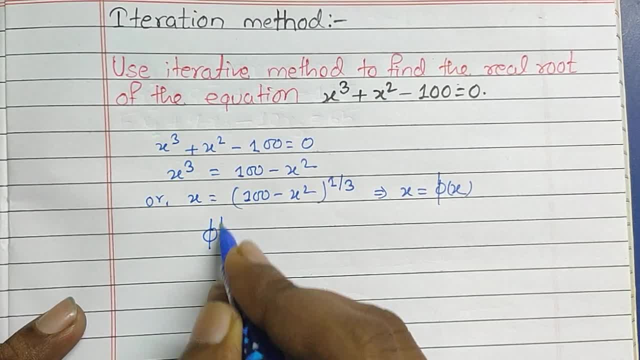 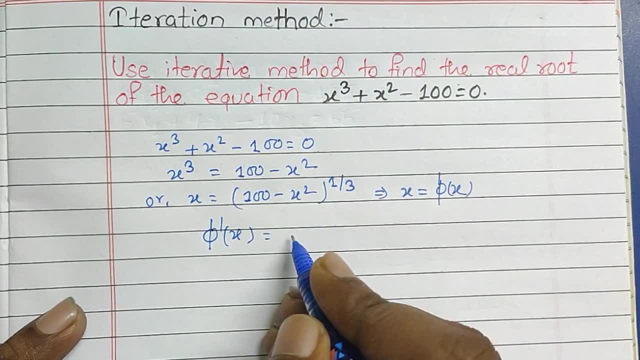 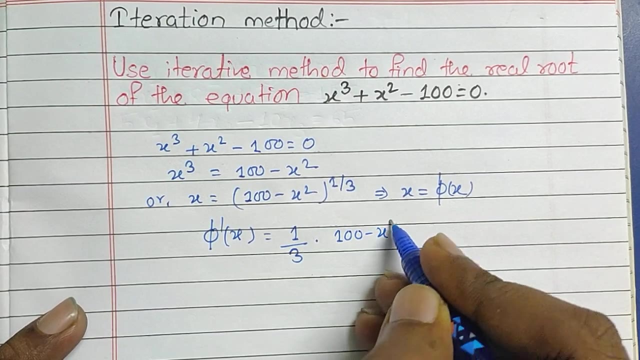 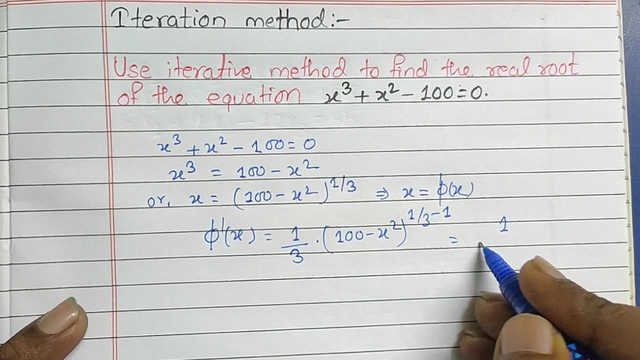 find its derivative. so its derivative is going to be 5. dash X is going to be 5. dash X is equal to 100 minus x square to the power 1 by 3. so its derivative is going to be N times x to the power 1 by 3 minus 1. so this is going to be 1 by 3. 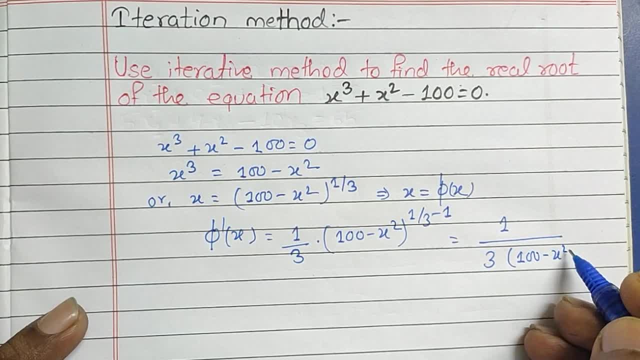 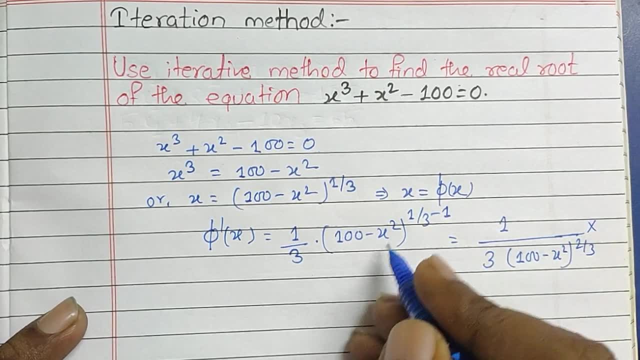 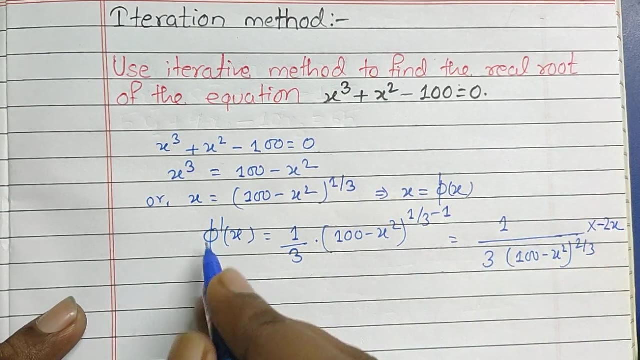 times 100. minus X to the power, minus x square to the power, 2 by 3 into this derivative of minus X square, will be minus to x. so we have got the value of phi dash x. now here i have got the value of phi dash x. 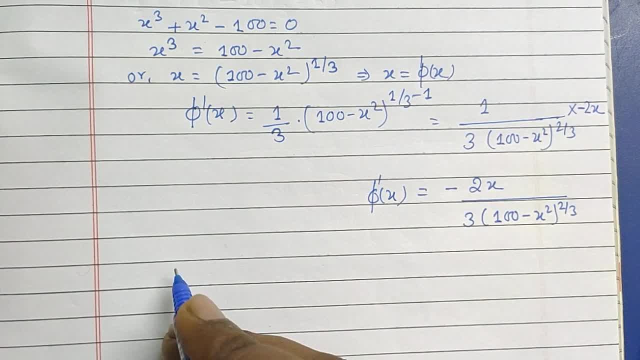 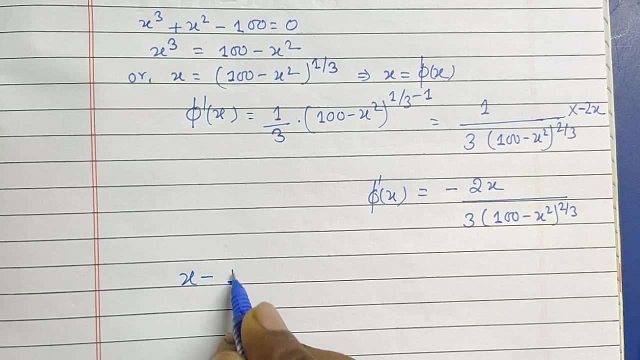 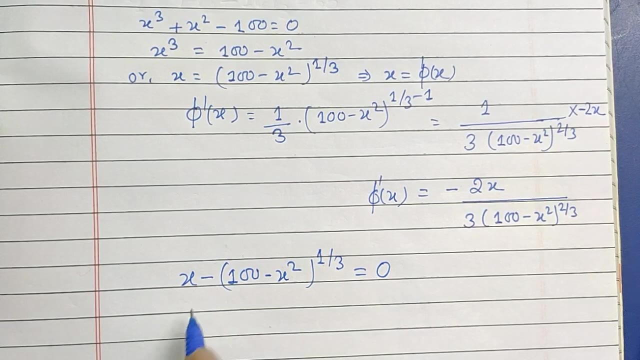 now what i need to do is i have to find the integer between which our value of x will lie. from here i can write that x minus 100 minus x, square to the power 1 by 3, is equal to 0. now what i will do is i have to put the value of x 1 by 1 from 1. 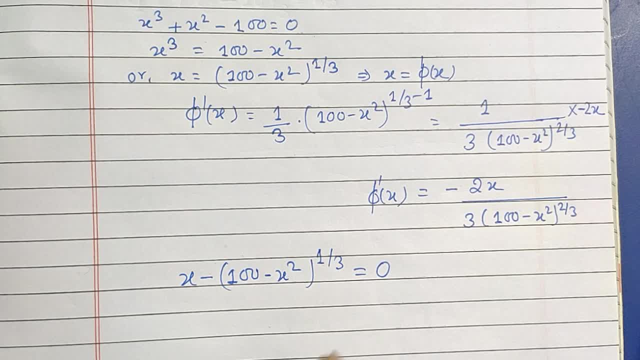 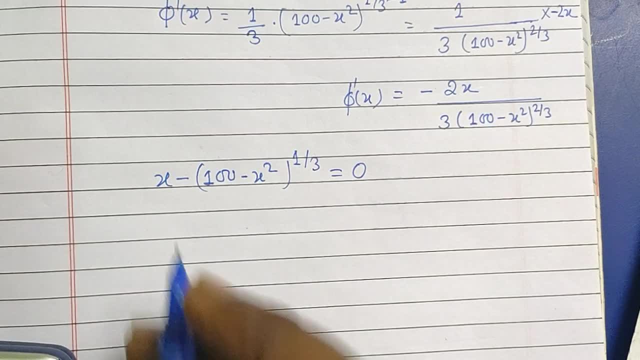 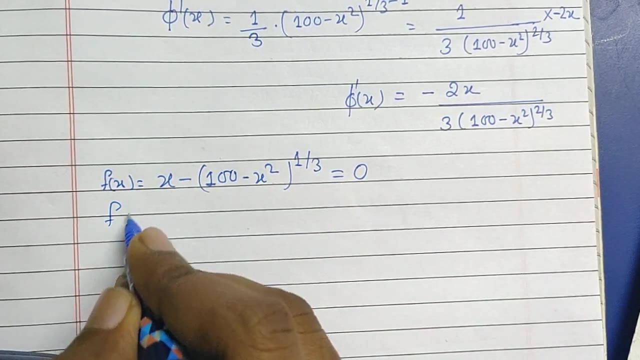 or 1, 2, 3, 4, like this, and then i will find a positive and negative value, and that will be our integer, between which our root will lie. as you can see, it can be written as: f: x is equal to x minus 100, minus x square to the power 1 by 3, so f1 is going to be 1 minus 100 minus. 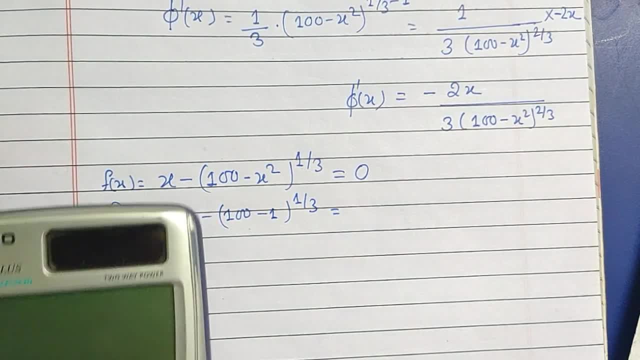 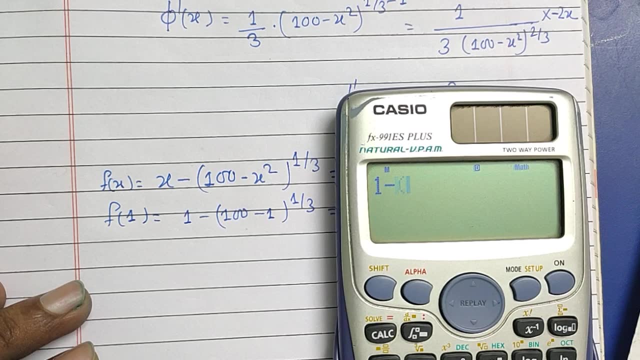 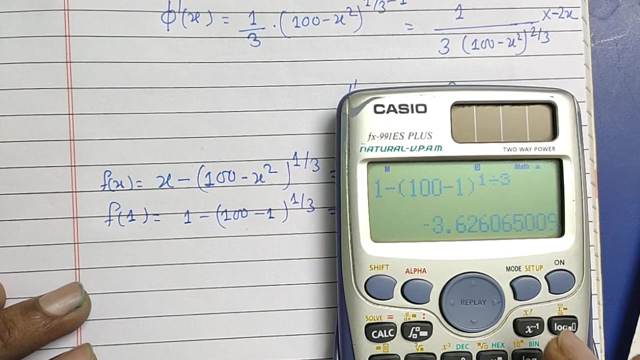 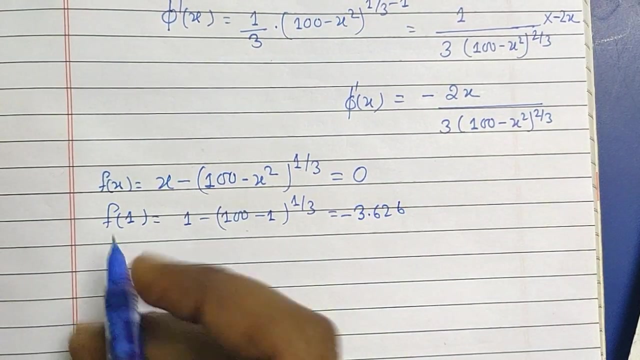 1 to the power 1 by 3, which will be solved by using calculator. so this is going to be 1 minus 100, minus 1 to the power 1 by 3, which is going to be minus 3.626. similarly, f2 is going to be. 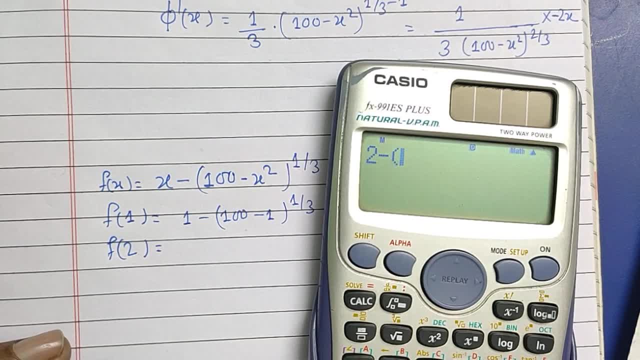 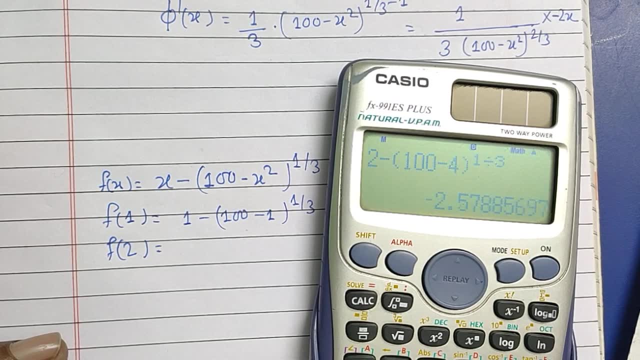 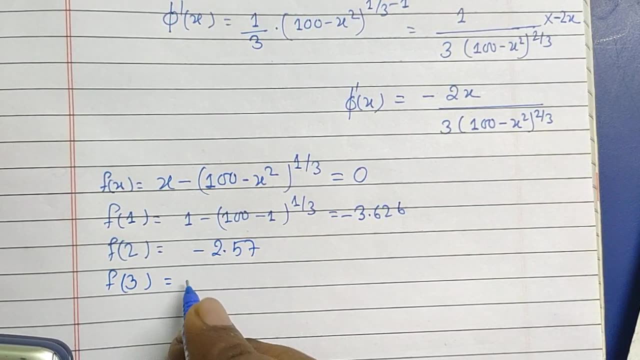 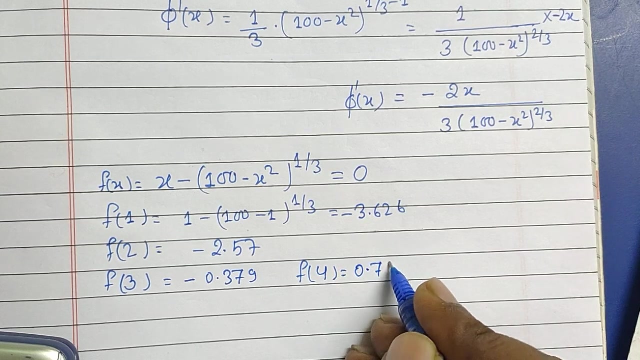 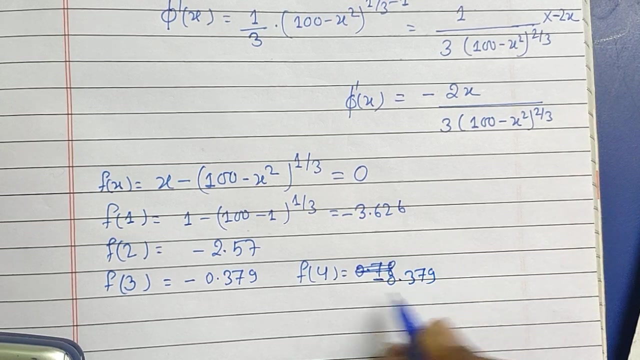 be 2 minus 100 minus 4 to the power 1 by 3, so this is going to be minus 2.57. similarly, f3 will be equal to minus 0.379 and f4 is going to be 0.78. sorry, f4 is going to be minus 0.379 and f3. 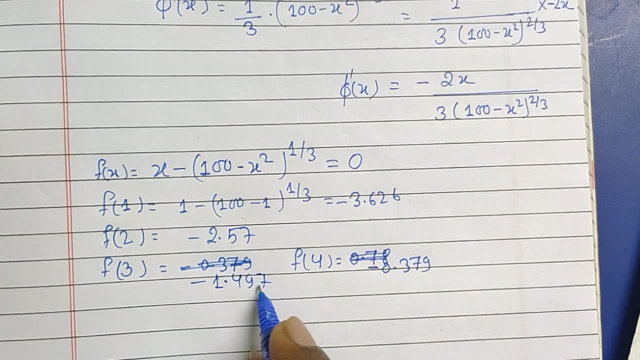 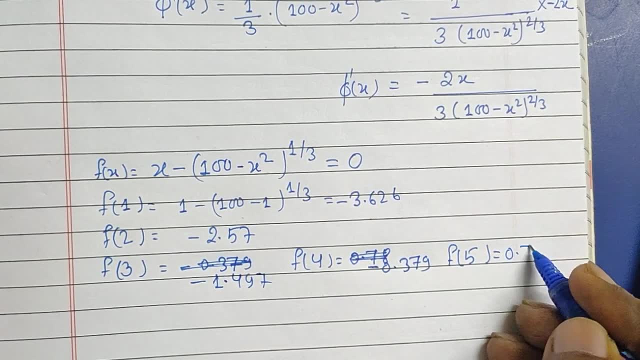 f3 will be minus 1.497, f4 will be minus 0.379 and f5 will be 0.78 means here i have got 0.379. and f4 will be minus 0.379 and f5 will be 0.379 means here i have got. 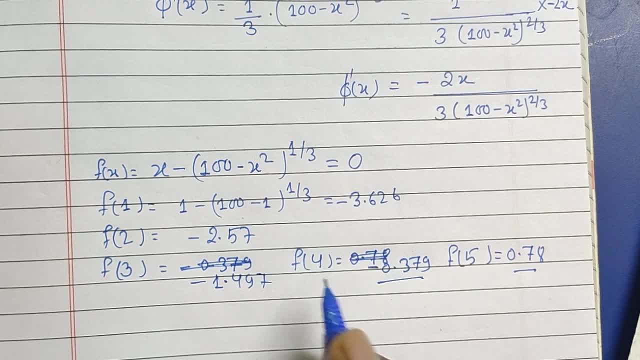 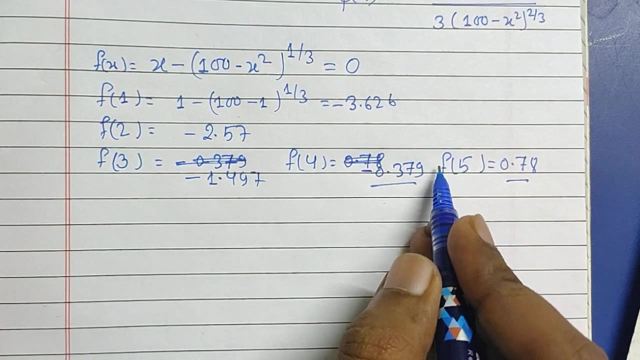 positive and negative value, which says that our root will lies between four and five, means i have got the integer i according to the theory of iteration method. now, after doing this, after finding the integer i, what we need to do is we have to check whether the iteration method is. 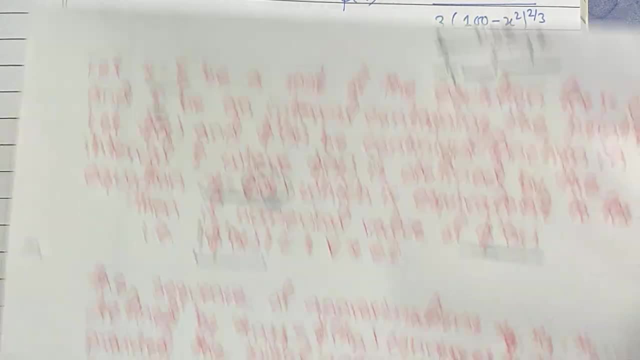 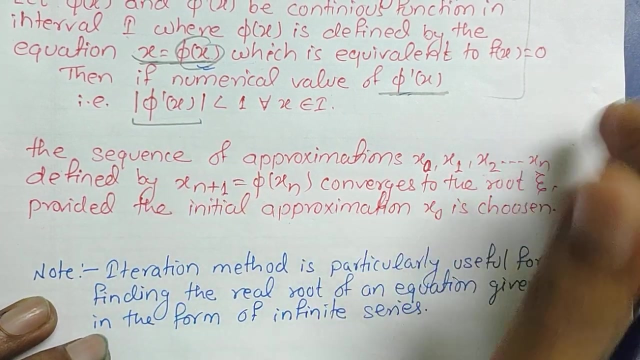 applicable or not and, as you can see, as per the theorem, it says that the iteration method is applicable only if the iteration method is applicable and if the iteration method is applicable, only if the iteration method is applicable and if the iteration method is applicable and if the iteration method is applicable and if phi dash modulus of phi dash x is less than one. 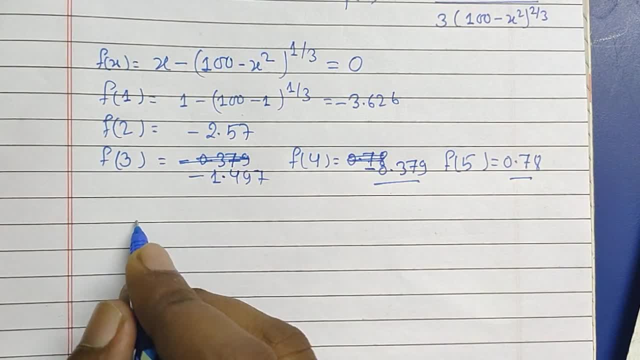 phi dash. modulus of phi dash x is less than one. phi dash. modulus of phi dash x is less than one means i need to find the modulus of phi dash x. so means i need to find the modulus of phi dash x. so means i need to find the modulus of phi dash x. so modulus of phi dash x. 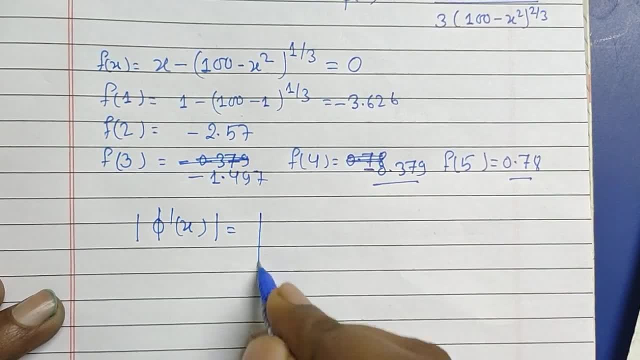 modulus of phi dash x. modulus of phi dash x will be equal to. modulus of will be equal to. modulus of will be equal to modulus of phi dash x. value is here: phi dash x. value is here. phi dash x. value is here here. this is phi dash x, so this will be. 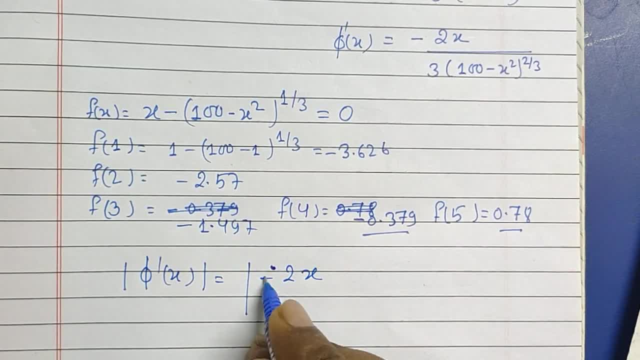 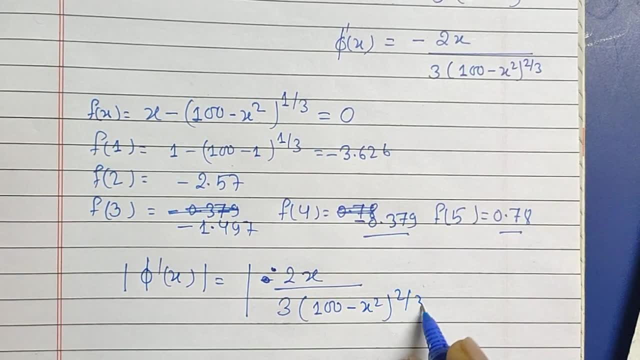 here. this is phi dash x, so this will be here. this is phi dash x, so this will be written as written. as written as minus two. sorry, this modulus will be become positive: 2 by 3, 100 minus x, square to the power 2 by 3, as we know that our root will lie. 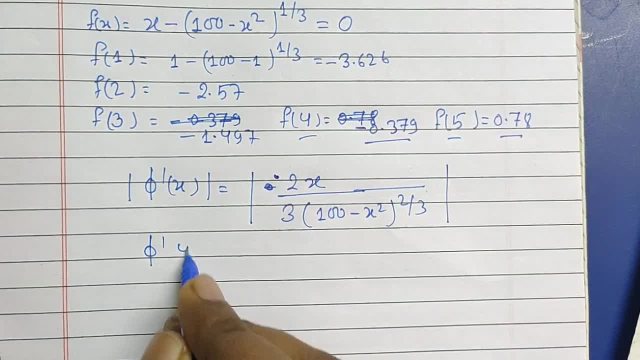 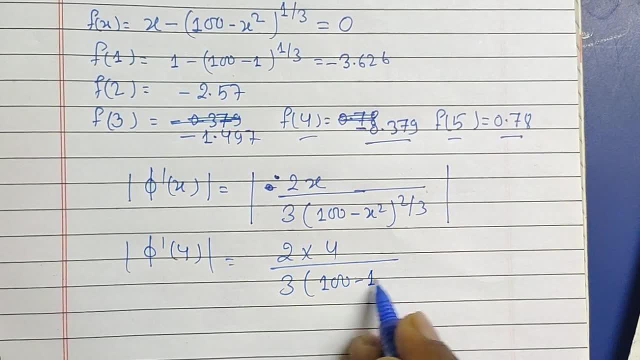 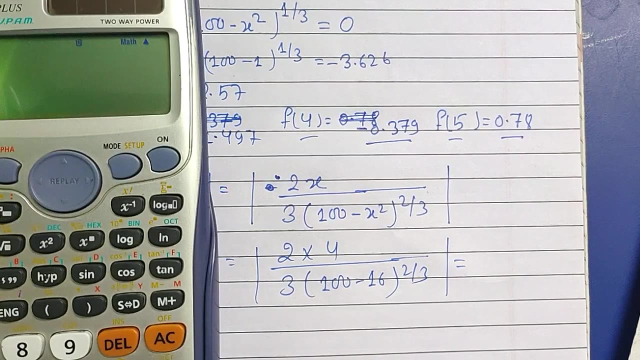 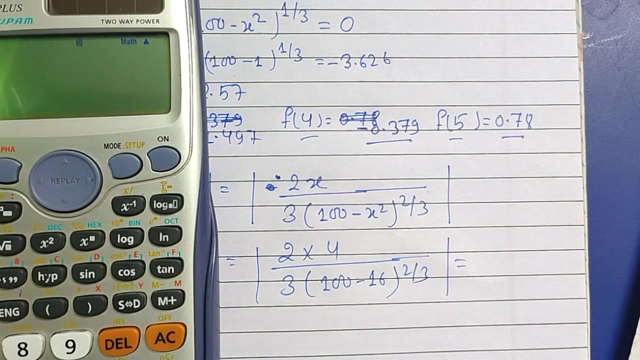 between 4 and 5. so 5 dash 4 is equal to 2 into 4 by 3 times 100 minus 16 to the power 2 by 3 modulus. so this is going to be 8 by 8 by 3 times 100 minus 16 to the power 2 by 3, and we have got. 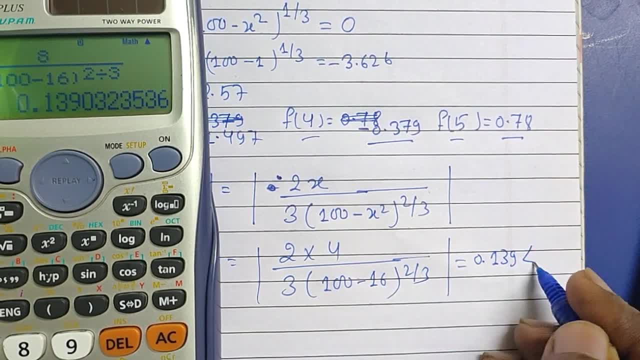 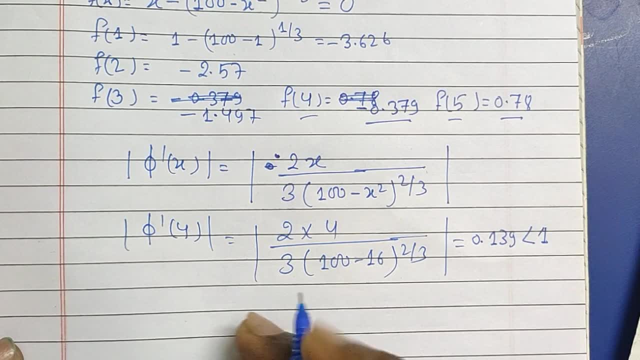 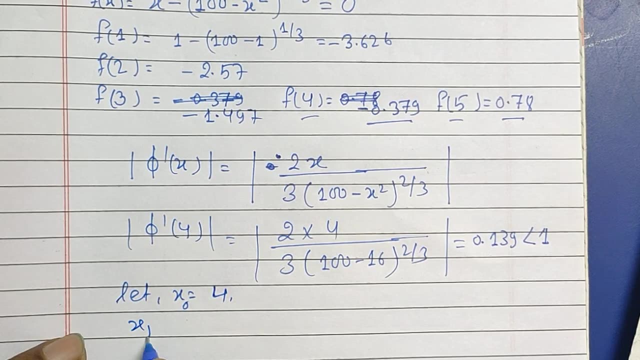 the answer, which is 0.139, which is less than 1, it says that iteration method can be applicable in this equation. so now let's take let x naught is equal to 4, so x1 is going to be, x1 is going to be phi x naught. 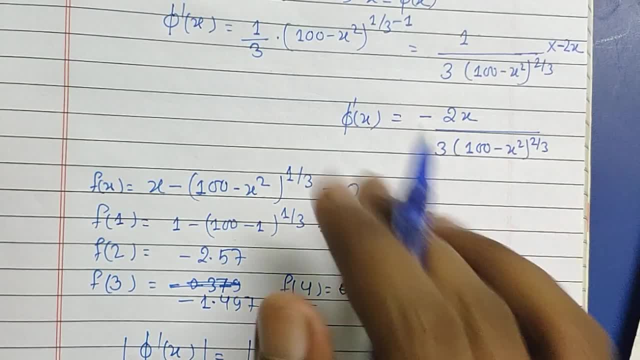 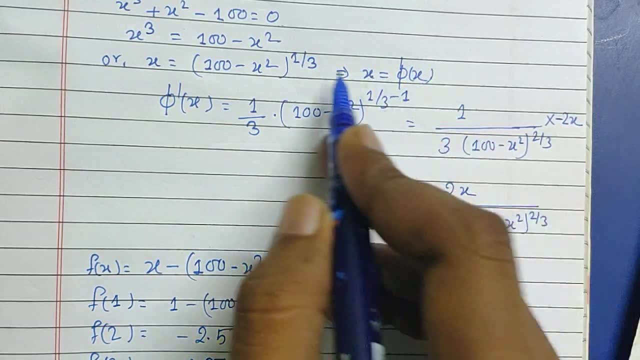 and we have got the value of phi x, phi x, and phi x is equal to 100 minus here, x is equal to phi x, phi x is equal to 100 minus x, square to the power 1 by 3. so here this is going to be. 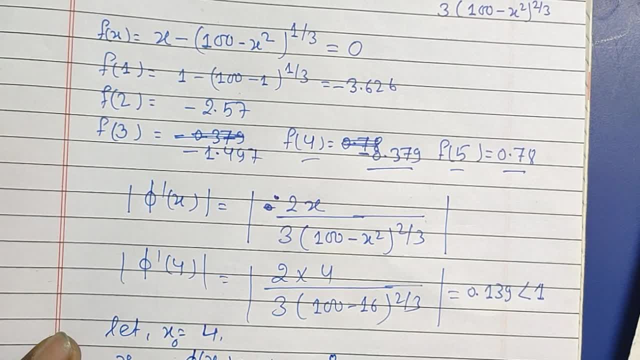 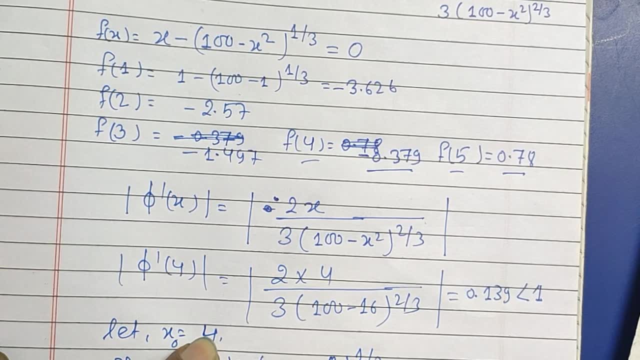 100 minus x naught square to the power 1 by 3, and we have got the value of x naught, which is 4. so 100 minus 16, this is 4 square 16 to the power 1 by 3, which is going to be. 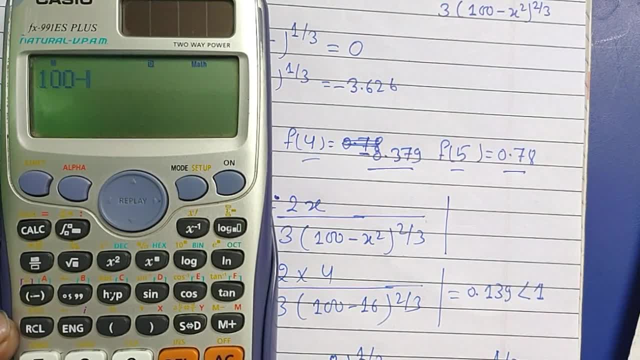 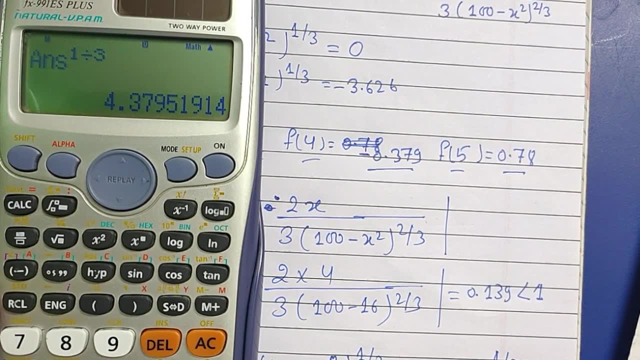 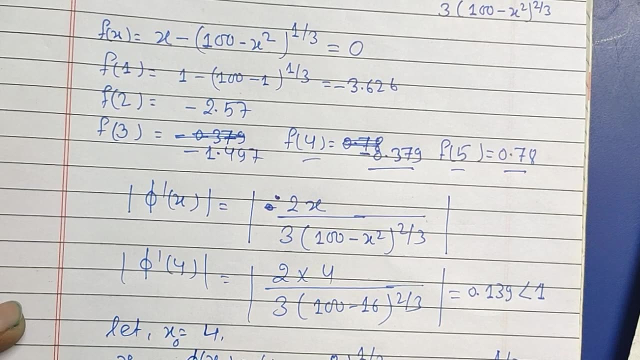 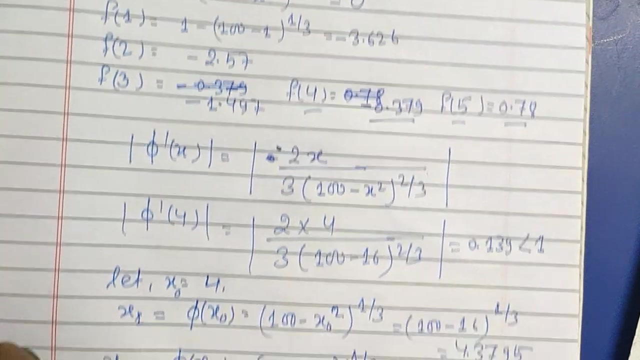 100 minus 16 to the power 1 by 3, and this is going to be 4.379 x2. this is going to be 5 x1, which is going to be 100 minus x1, square to the power 1 by 3, and 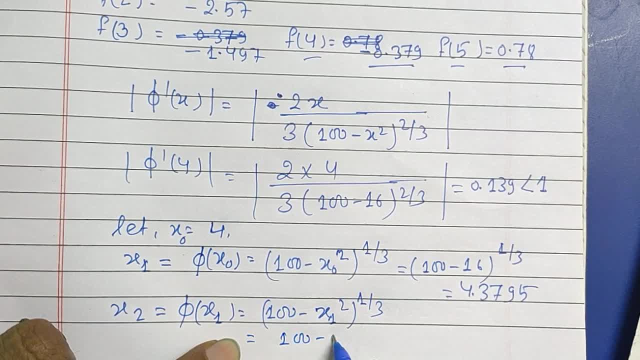 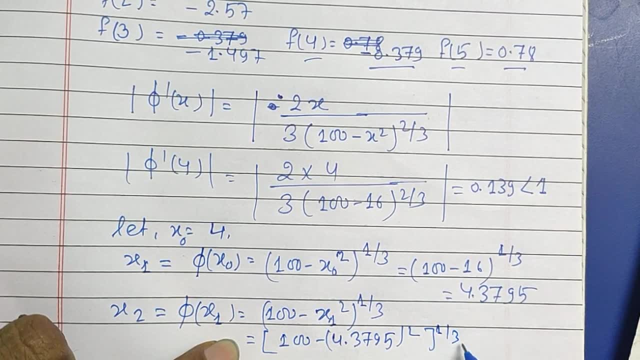 here this is going to be. 100 minus x1 means 4.379, 5 square to the power 1 by 3. on solving this, you will get 100 minus 4.379, 5 square to the power 1 by 3, and here this is going to be. 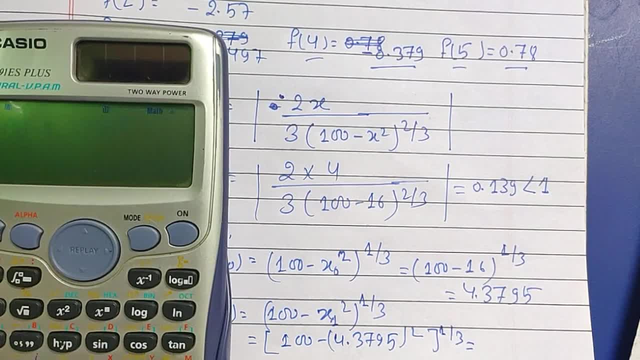 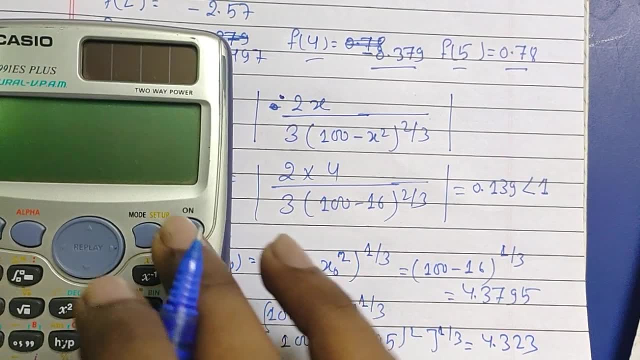 4.379, 5 square to the power 1 by 3, and here this is going to be 4.379, 5 square to the power 1 by 3, which will be equal to 4.323. similarly, uh, we have to proceed for x3, x4 until we get the two to three digit after decimal. 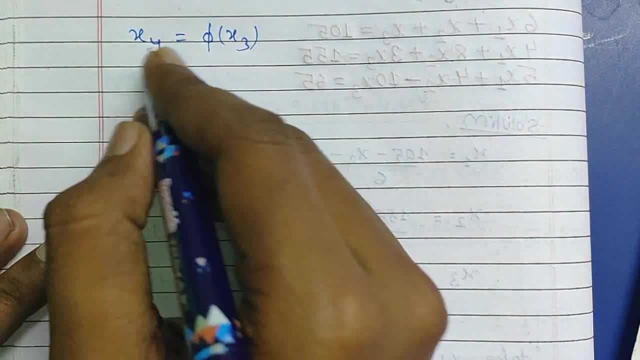 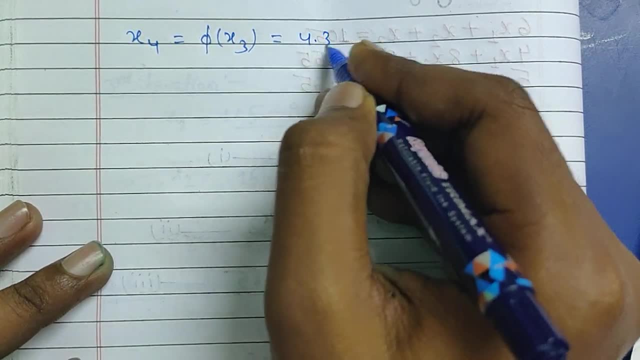 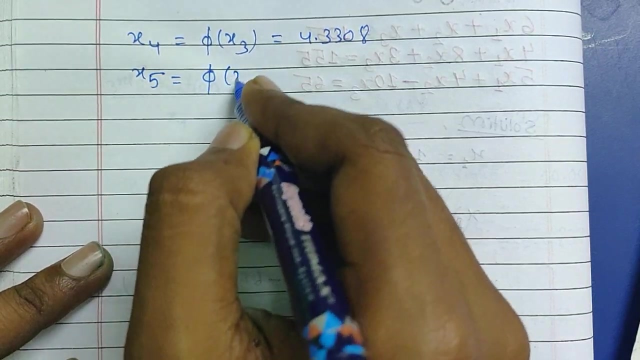 same and that will be our. similarly, x4 is equal to 5 x3. so put the value of x3 in that equation you will get four point three, three zero eight. four point three, three zero eight. four point three, three zero eight. and this is our x4. find x5. x5 will be equal to 5, x5, so put the value of x4. sorry, here it will be x4. 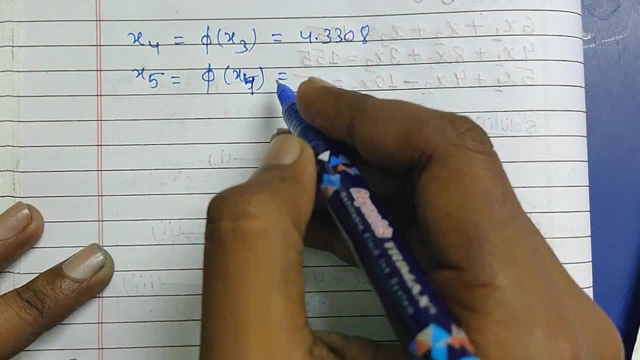 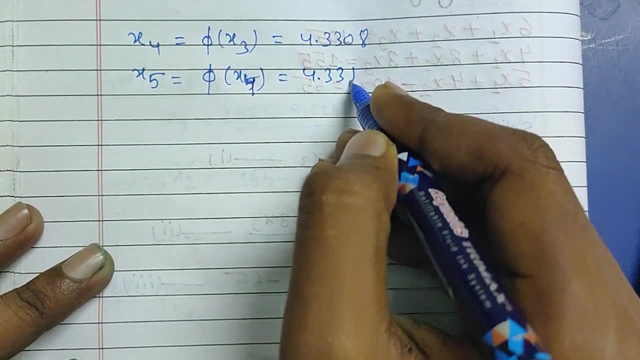 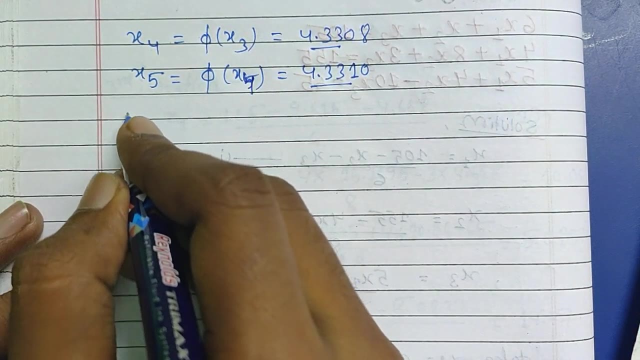 so put the value of x4 in that equation which i have shown in the x2, and x1 and x3 also, so you will get 4.3310 and, as you can see, after decimal we are having two digit, two digit similar, since we can say that the 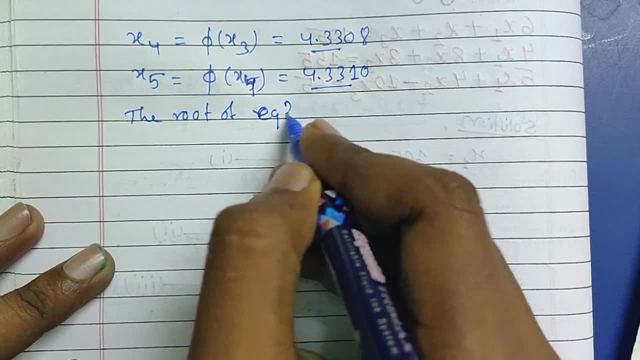 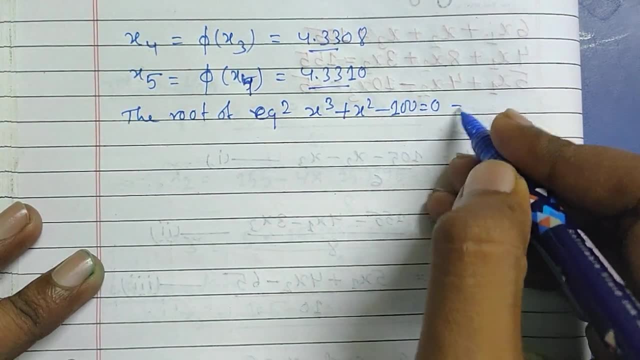 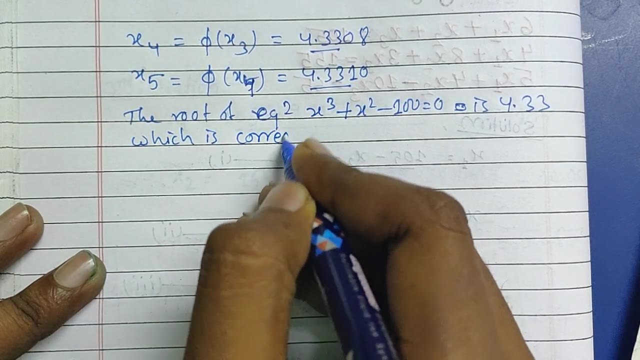 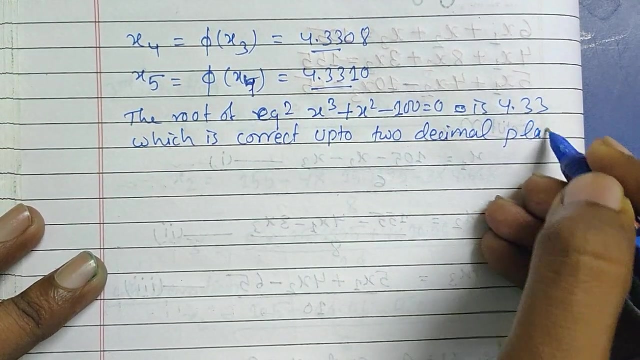 root of equation x cube plus x square minus hundred is equal to zero. is is four point three, three, which is correct, up to two decimal place here, and this was the final answer of this. this was the final answer of this. this was the final answer of this. 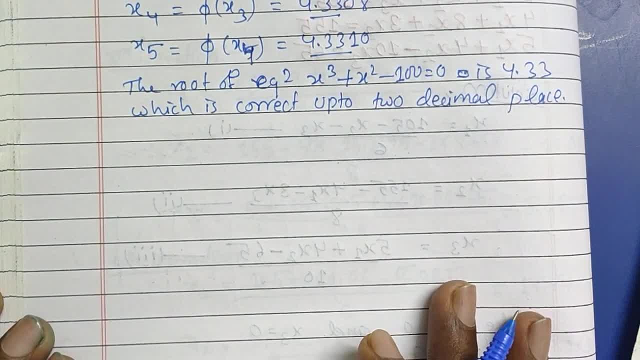 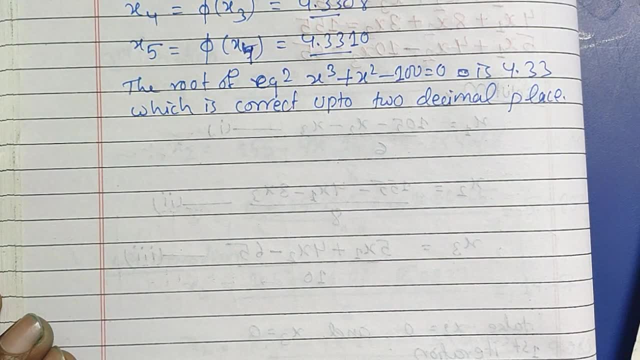 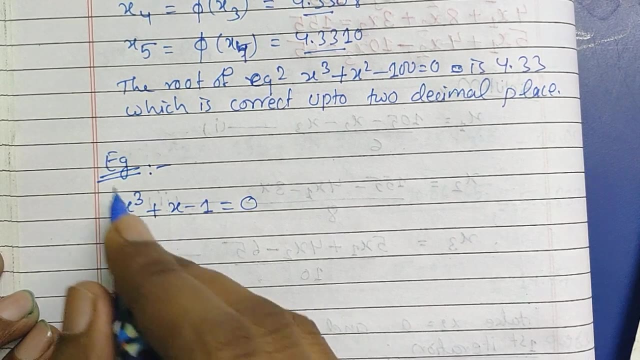 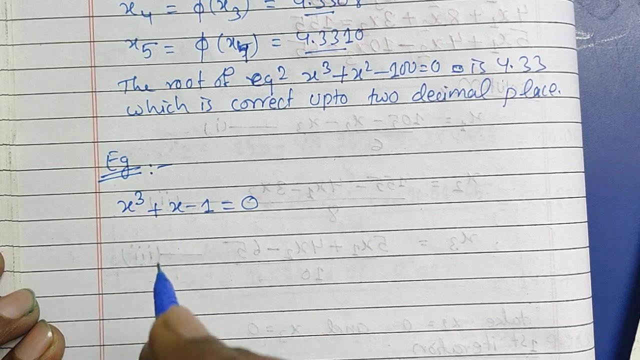 question and, students, let me take, make you clear that, why i arrange this equation in to find the rule to find the phi, dash x should be less than one, why i have done that here. that thing, that is the thing, and that i have the white dawn while solving this numerical. i am going to make you clear by using this question. 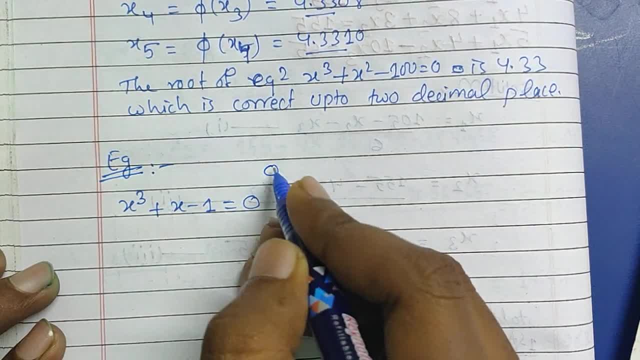 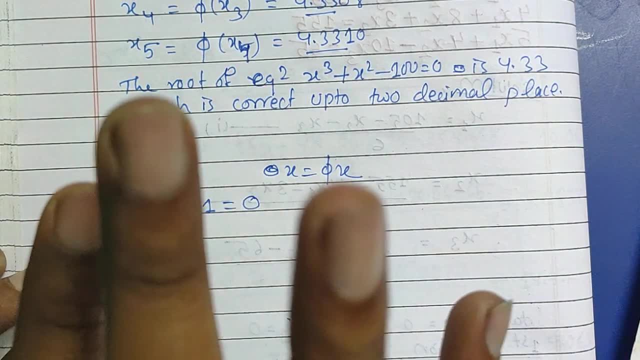 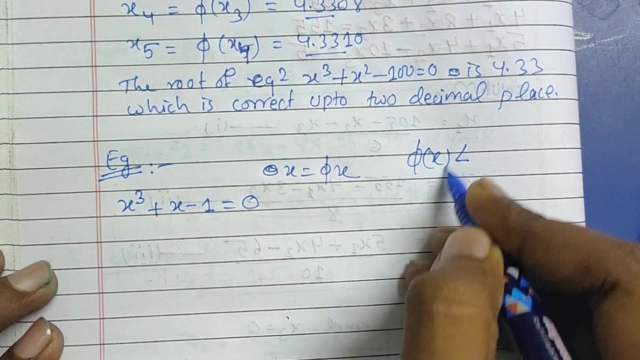 see, here i am going to write this equation in, in the form of: x is called to five acts and c it can. this equation can be written in three ways, and out of which only of one. one equation will be valid for five. dash x is less than one, and i will show you that. see, i can write it at. 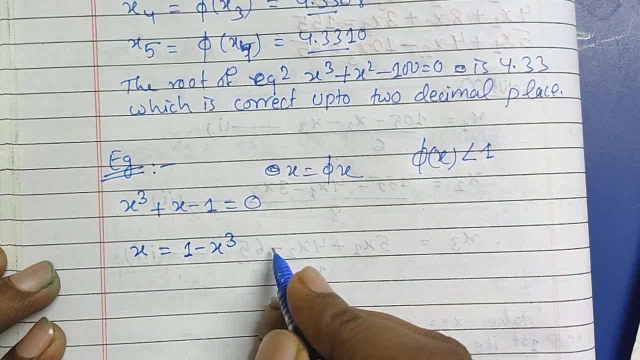 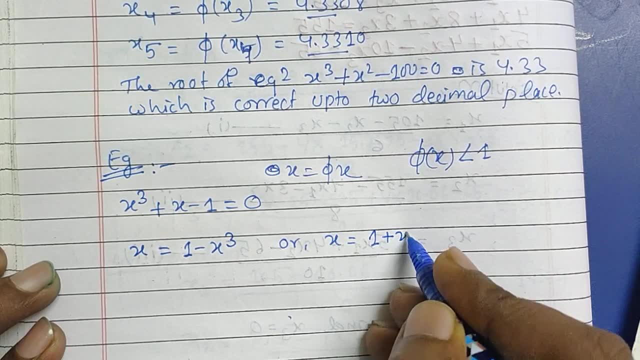 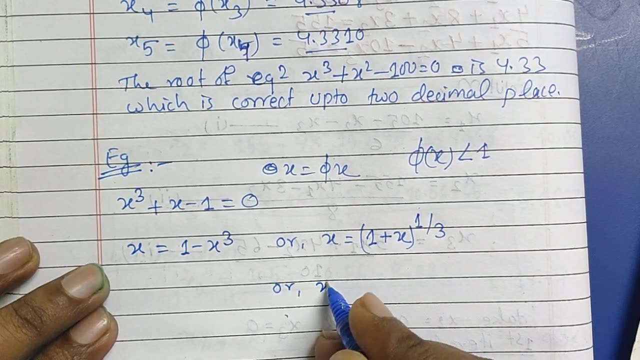 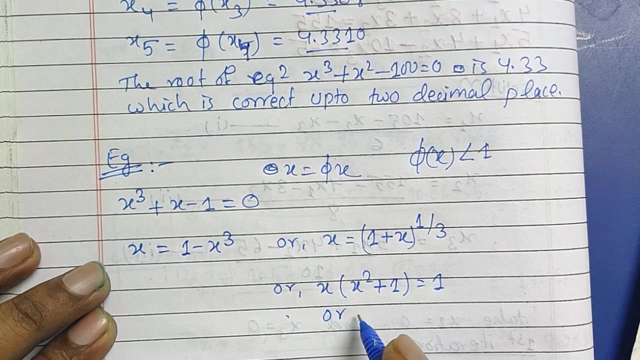 x is equal to one minus X, Q or x is called to one plus x to the power and x is equal to two 1 by 3 or x times x. square plus 1 is equal to 1 or x is equal to 1 by x. 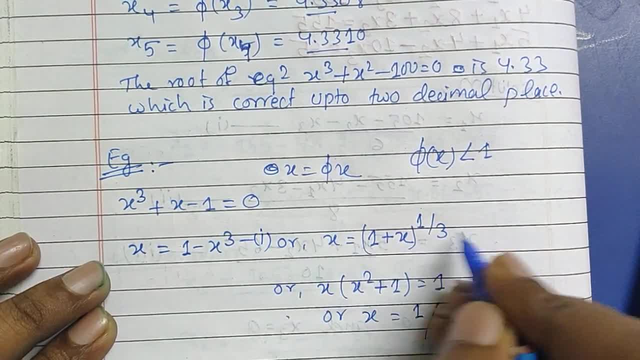 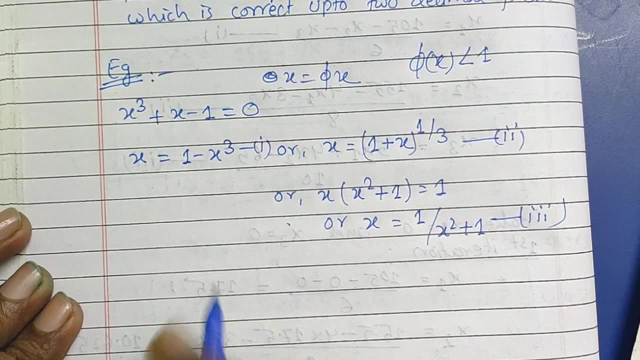 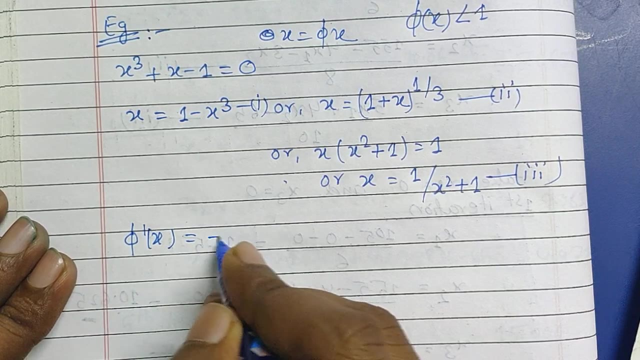 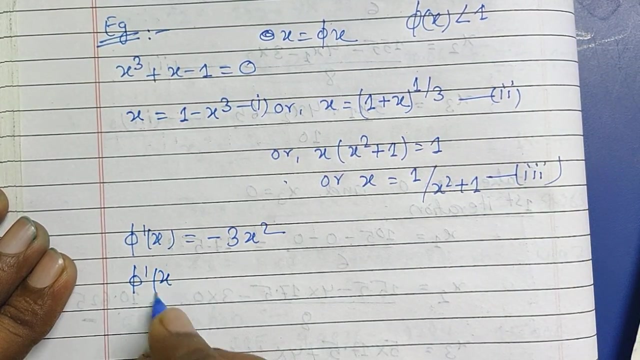 square plus 1. this is our equation 1. this is our equation 2. this is our equation 3. now on, taking the derivative of first equation, phi dash x, will be equal to minus 3 x square. derivative of second equation, phi dash x, will be equal. 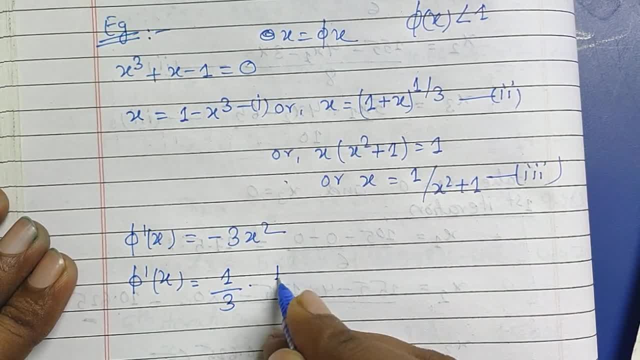 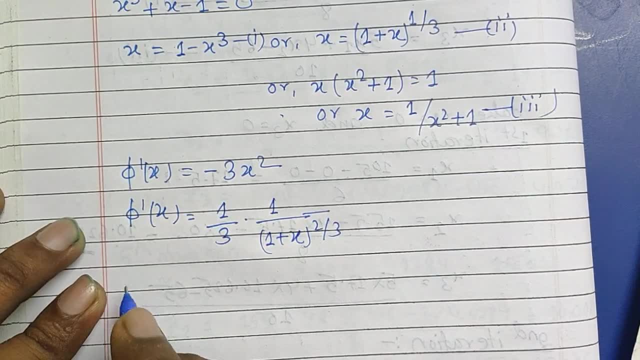 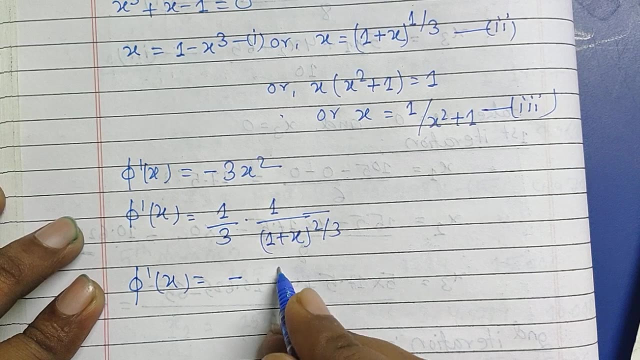 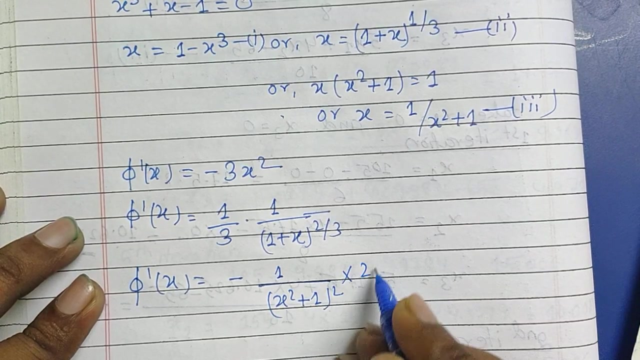 to 1 by 3 times 1 by 1 plus x to the power 2 by 3. similarly, derivative of third equation, phi, dash x is going to be minus 1 by x, square plus 1 to the power 2 into 2x. now, 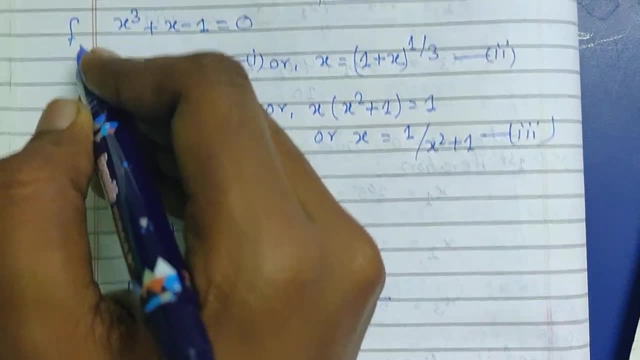 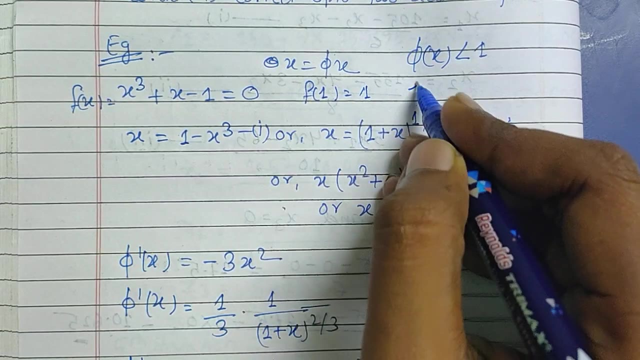 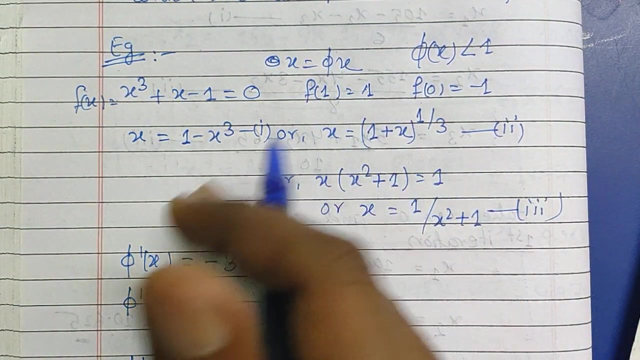 and here, as you can see, that fx is equal to this. so f1 will be 1 and f0 will be minus 1. so we all know that our root of the solution of the, of the root of the equation, will lies between 1 and 0. as you can see, if I will find the modulus of: